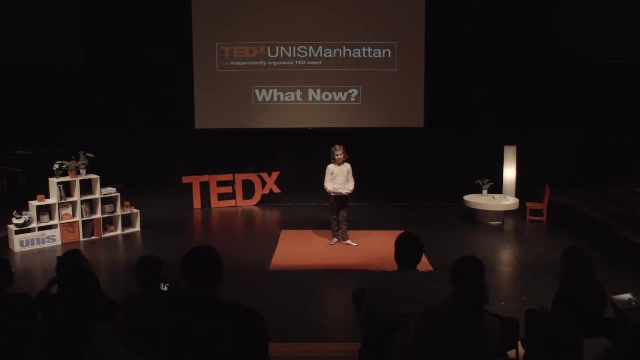 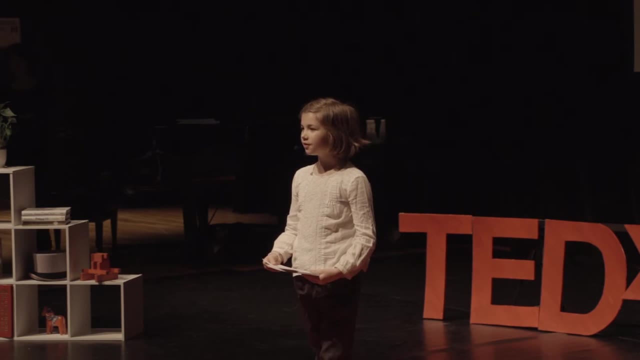 My name is Talam Balefolk and I am in the fifth grade, And, besides the United States, I have lived in Kenya, Ghana and Rwanda. Today, I would like to attend the University of Geneva to become a lawyer or a politician. 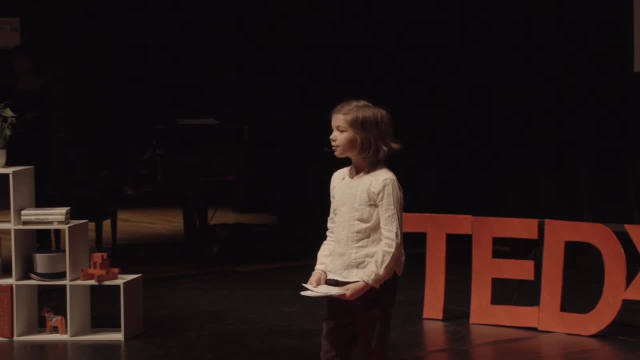 But today I will talk to you about how to use sports to improve the lives of kids. According to the 2016 Statistic Brain Research Institute, 60% of kids in the United States play sports outside of school. I would like to see that percentage go to at least 90%, because if kids use their energy productively, 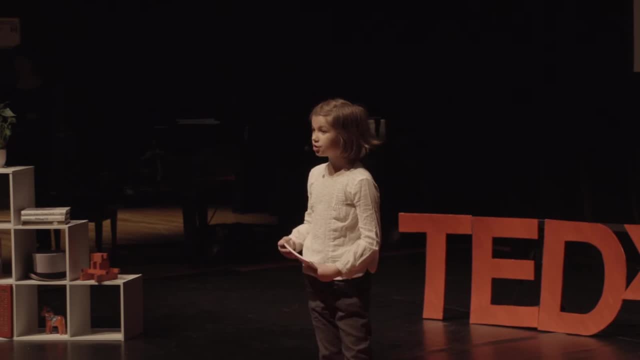 they may not have time for unhealthy behavior That could lead to joining gangs, playing mindless video games or becoming a couch potato. We can help us kids who are at risk by encouraging ourselves and our friends to get involved in a sport. According to the Power Supply Unit Education, kids who play sports in school often enjoy social interaction better. 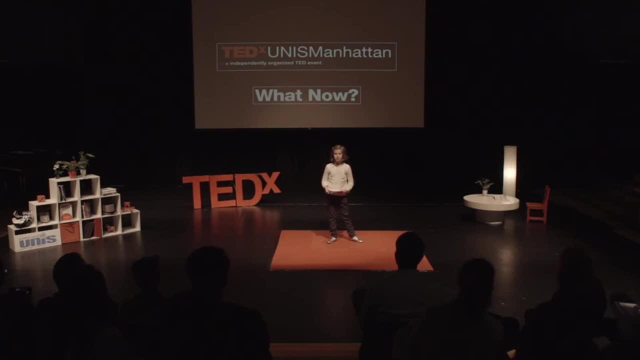 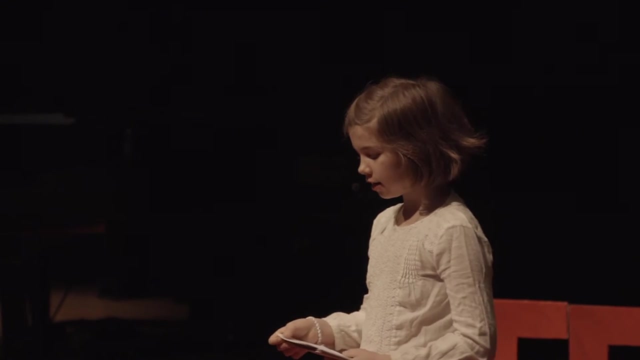 Participation in sports by children and teens is associated with a range of factors. Participation in sports by children and teens is associated with a range of factors. They have documented physical, emotional, social and educational benefits. Professor Margaret Tablad, president of the International Council for Sports Science and Physical Education. 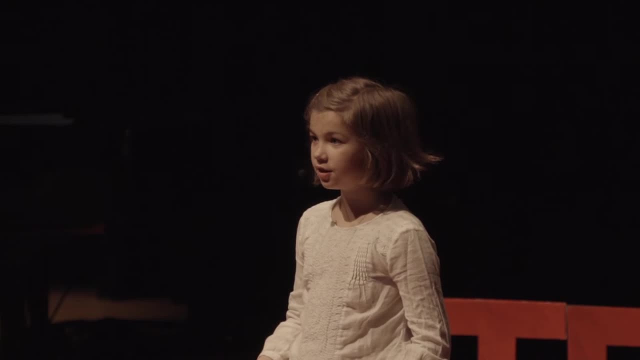 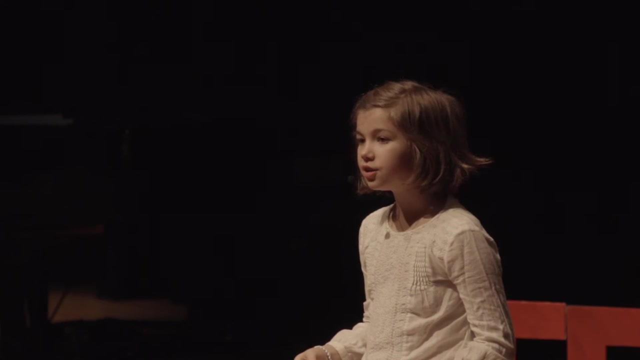 once wrote that dance and other challenging physical activities have a huge impact on the self-esteem of kids. So dance, gymnastics, hockey and volleyball can teach children to enhance their potential in new ways. Did you know that sports can even help kids make friends? 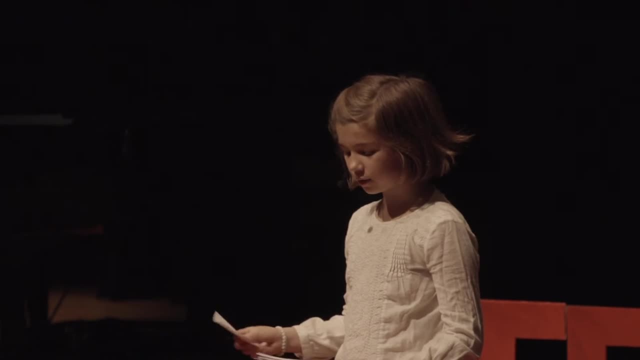 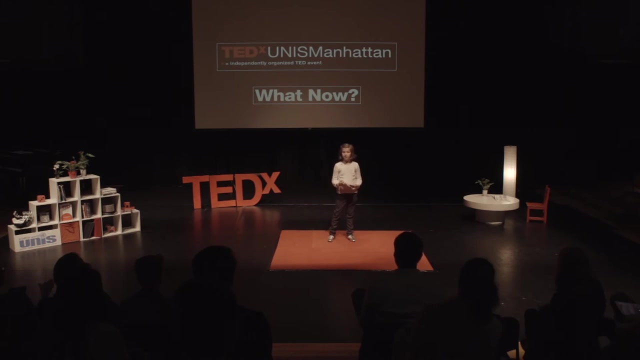 Because, according to the National Association for Sport and Physical Education, kids who play sports in school often enjoy social interaction better. In her book Run Like a Girl, Mina Samuel explains: over the years that followed my discovery of running, my self-confidence grew. 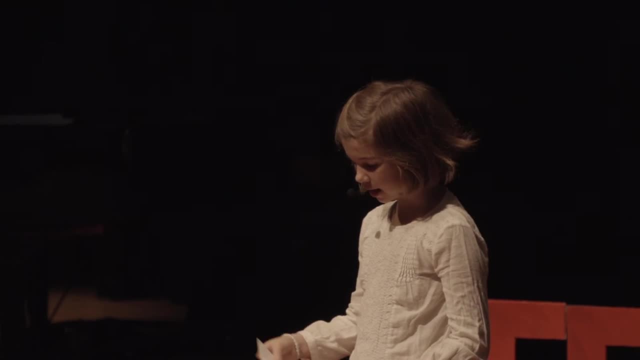 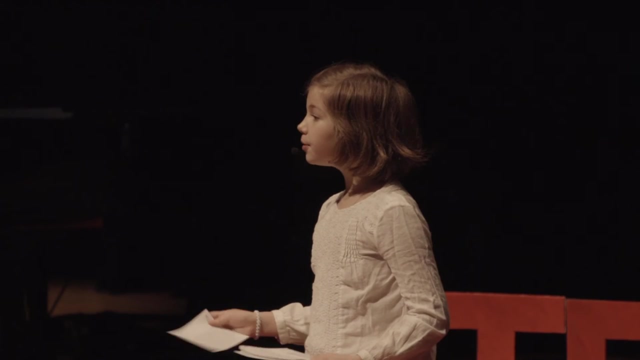 I discovered a capacity within myself that I never knew I had. I saw that I could push myself and take risks, not just in sports, but elsewhere too. The competition, in sports, as in life, was not with myself, It was not with someone else, it was with myself.